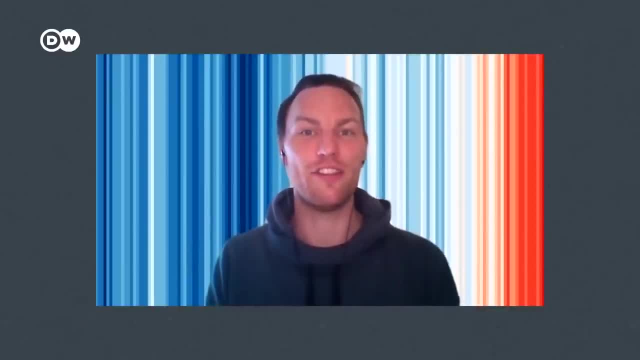 The fact that we are nowadays living in a world which has like oxygen in the atmosphere is mostly due to the so-called great oxygenation event, which is when, about a couple of billion years ago, cyanobacteria started producing oxygen and thereby created the world we live in today. 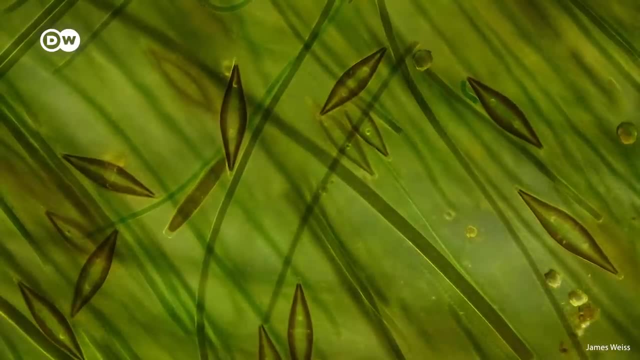 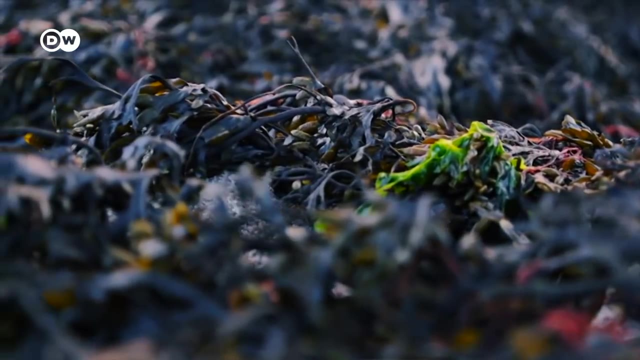 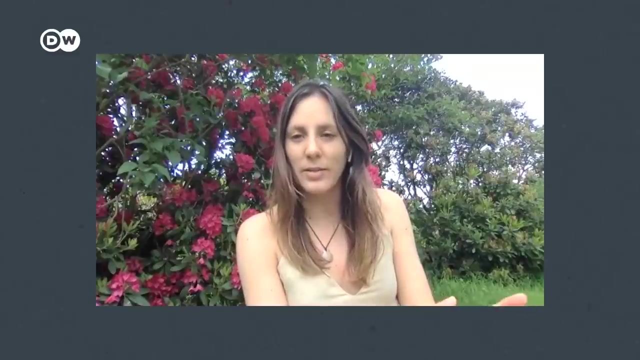 Cyanobacteria are what are called microalgae- Very small Macroalgae, on the other hand, is what washes up on the beach and what many call seaweed. Algae are actually like the plants in the ocean, And so they do the same process as plants do on land. 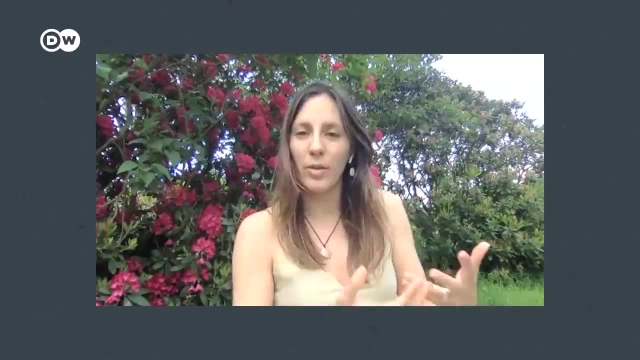 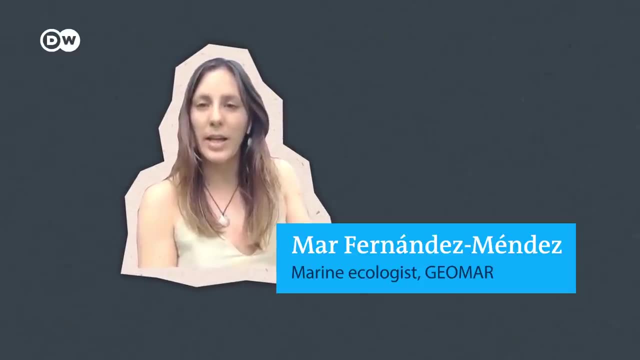 which is photosynthesis, So they take up CO2 and they convert it using sunlight. This is Mar Fernandez-Mendez. She's a marine ecologist studying how algae capture carbon and impact the whole marine food chain When an algae uses up that carbon from the ocean. then the ocean immediately absorbs carbon from the atmosphere because it's in constant equilibrium. So if you remove something, it needs to get equilibrated with the atmosphere again. Ocean algae absorb one quarter to a third of global CO2 emissions every year, But all algae do this even if they aren't in the ocean. 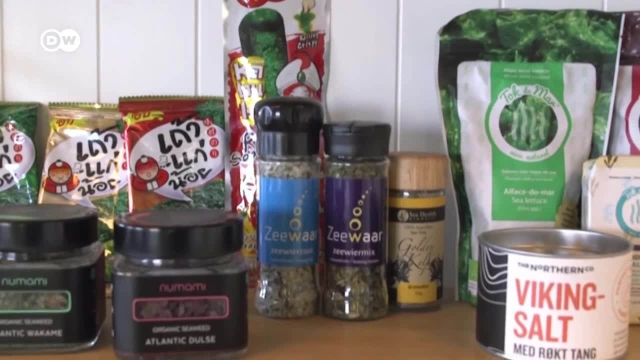 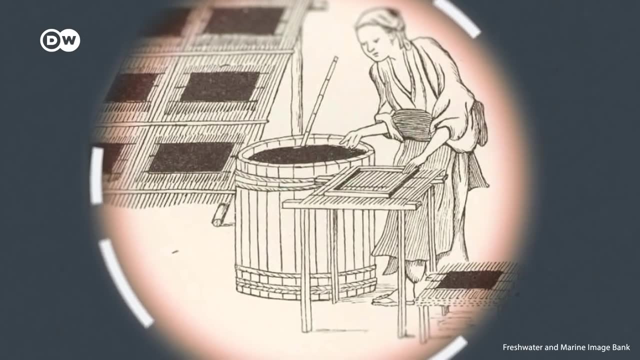 So, no matter what it's used for growing, algae captures CO2.. And humans have been using algae for thousands of years. Indigenous peoples from the Americas to East Asia are the original seaweed farmers. Seaweed was even mentioned in the oldest known Japanese poetry. 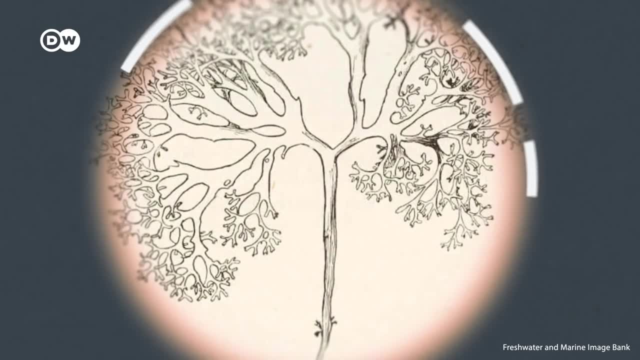 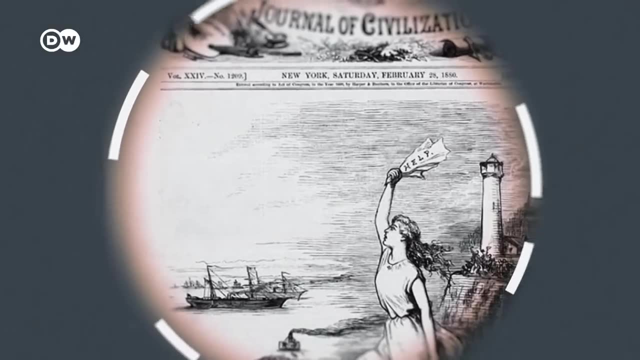 From Ireland. a type called Irish moss is used worldwide as the food additive. carrageenan Algae also helped people there survive the Great Famine of the 1840s. Today, algae aquaculture is most well developed in Asia, where it makes up a large part of the cuisine. 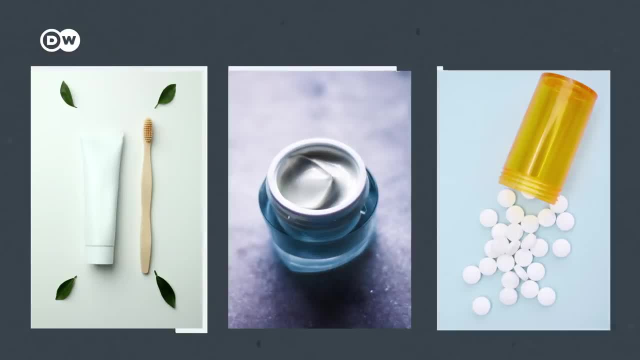 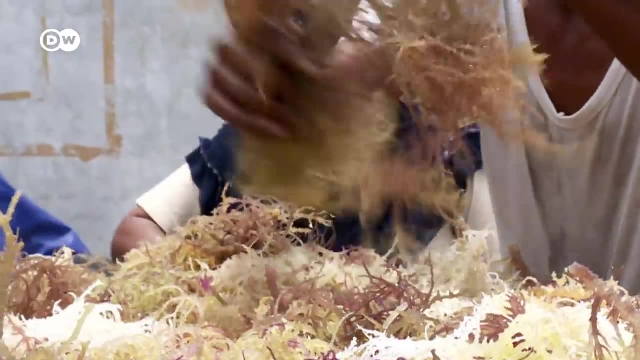 It can also be in toothpaste, cosmetics and medication. Growing algae for these products captures CO2,, but greenhouse gas reduction is not the main aim. That's about to change, because using algae as animal feed, fertilizer and bioplastic 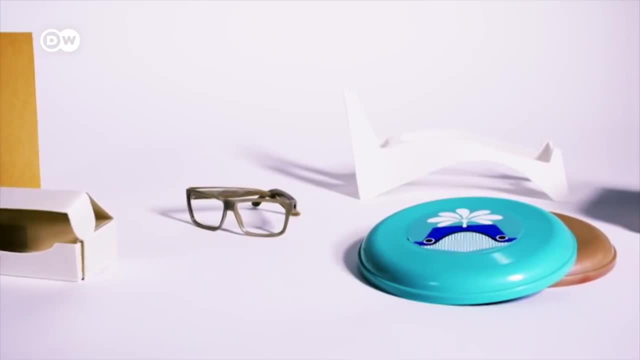 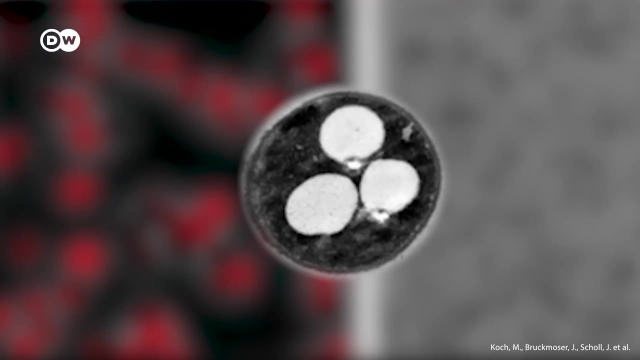 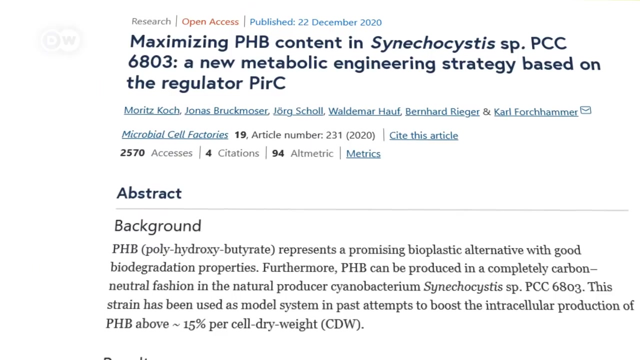 also diverts emissions from polluting industries, Its impact has effectively doubled. Let's talk about plastic. Some algae naturally contain and produce a bioplastic called PHB. It can replace polypropylene, the second most widely used traditional plastic, In this landmark paper. 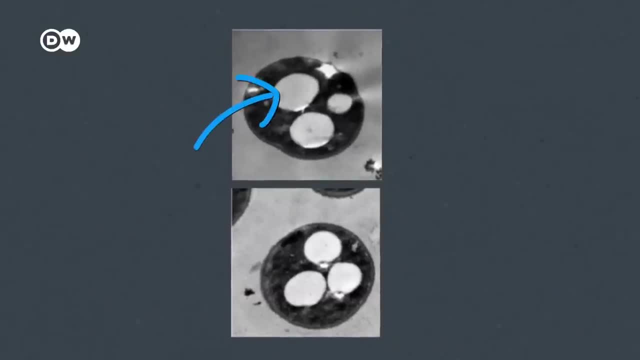 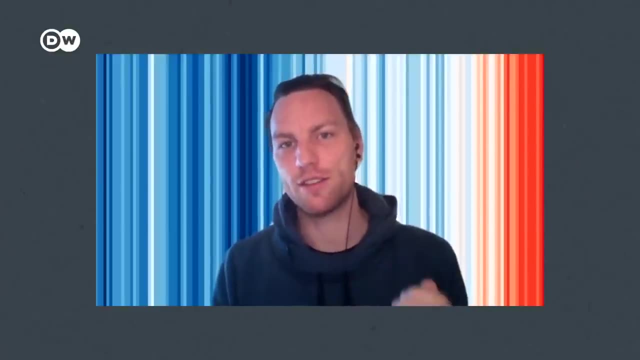 Weitz and other researchers modified blue-green microalgae, or cyanobacteria, to produce more of it. Using some metabolic engineering techniques, we were able to increase this amount from 10% to more than 80%, So we really created almost like true bioplastic bacteria. 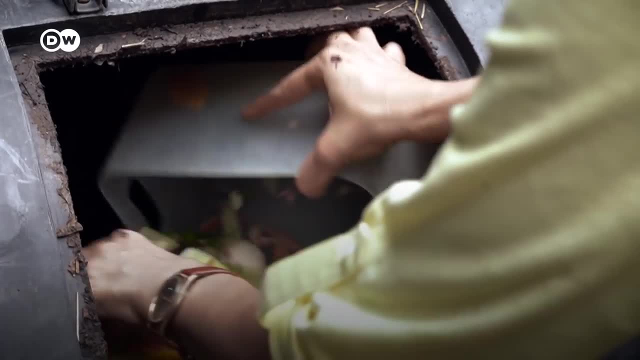 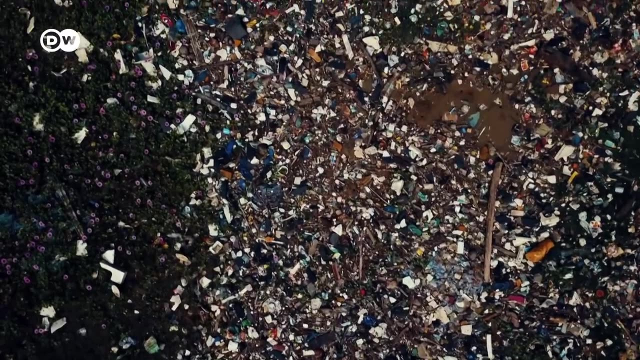 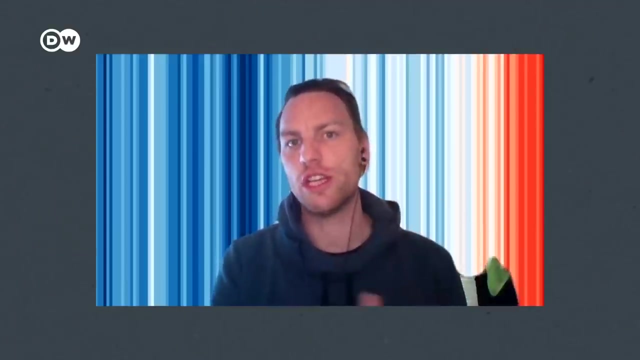 which consisted mostly out of bioplastic. PHB disintegrates under normal household compost conditions and releases no pollutants into the environment, unlike other bioplastics, And we already have the infrastructure to produce it. You could essentially already use the existing technology. 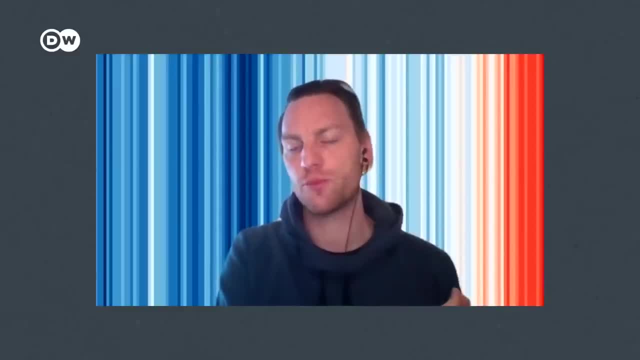 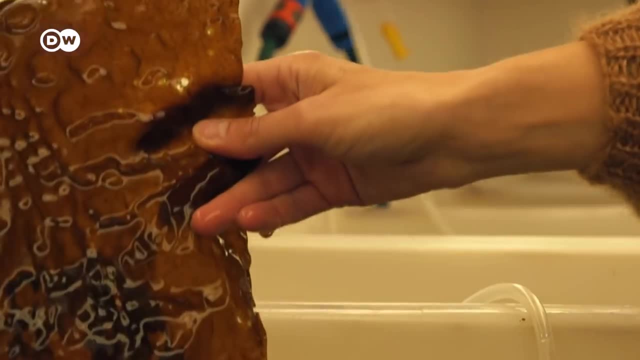 for producing different cyanobacteria, not just for food consumption, like spirulina, but also for the production of bioplastics, for example. Aquaculture technology can also be used to grow macroalgae, And one type has a truly amazing property. 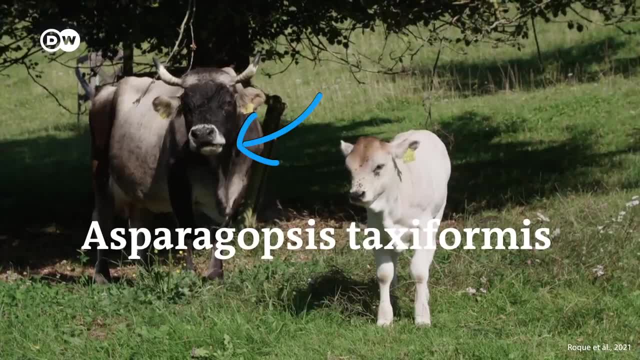 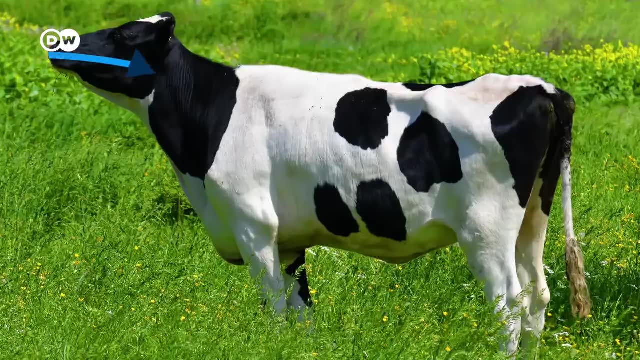 When asparagopsis taxiformis is added to animal feed, it reduces methane from livestock by up to 82%. Methane is produced in the stomach of livestock during digestion, which the animals then release. Compounds in this seaweed appear to stop the gas. 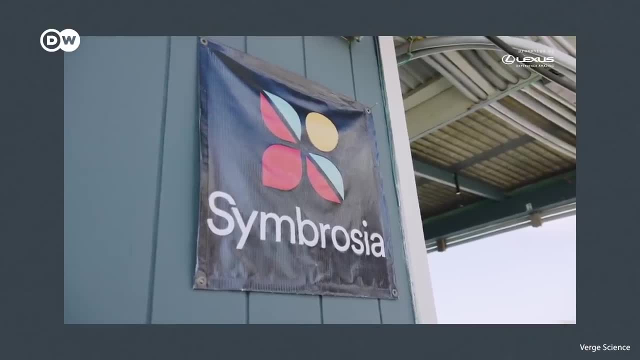 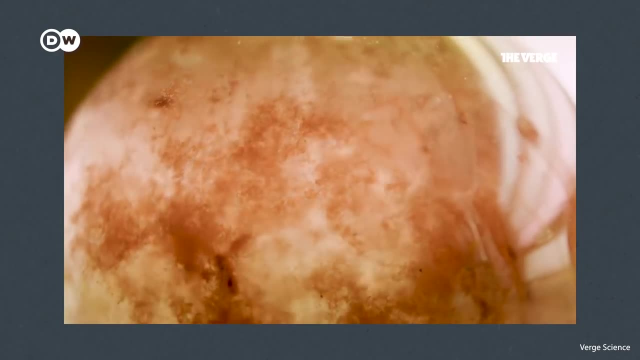 from forming in the first place. Startup Symbrosia is in the media spotlight for producing algae feed for livestock, But questions remain as to scalability, partly because this algae needs to be farmed. In some cases, however, the algae is already there. 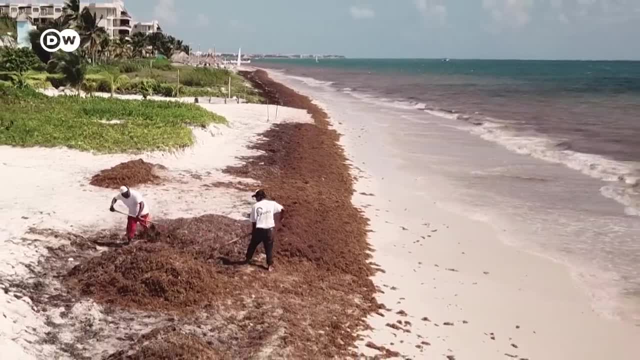 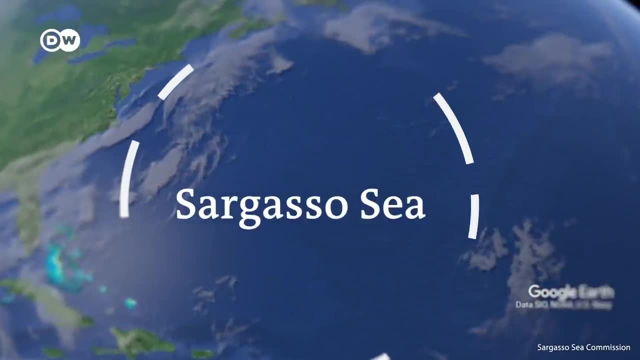 like sargassum, a perfect example of too much of a good thing. Its home is the Sargasso Sea, which accounts for 7% of the CO2 absorbed by all the oceans, But due to global warming and pollution, sargassum is growing out of control. 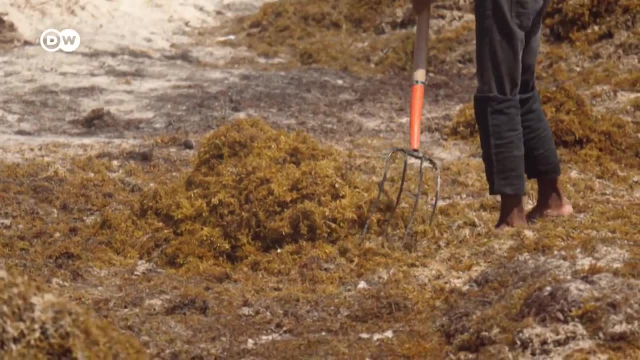 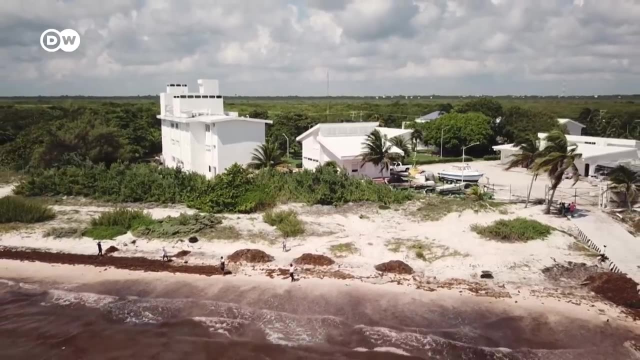 Huge amounts are washing up yearly in the Caribbean and Gulf of Mexico. In 2018, the bloom weighed over 20 million tons. Normally the algae would disintegrate, but now it's washing up onshore. Besides smelling horrendous, it contaminates the water. 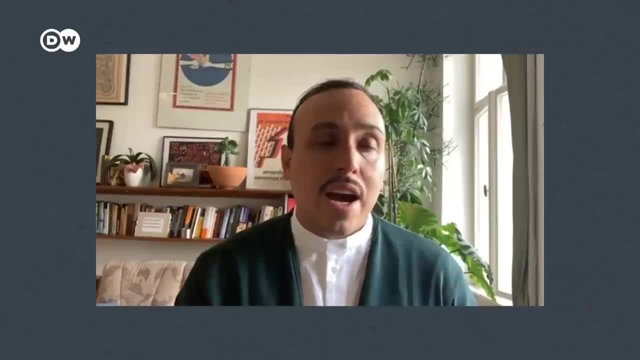 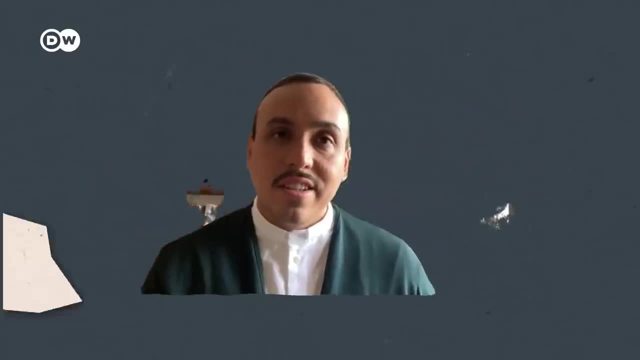 killing off animals and destroying coral. At this quantity, these mats of sargassum are basically death stars. Jorge Vega Matos works at Sea Combinator, a company that focuses on using sargassum blooms to make climate-friendly products. 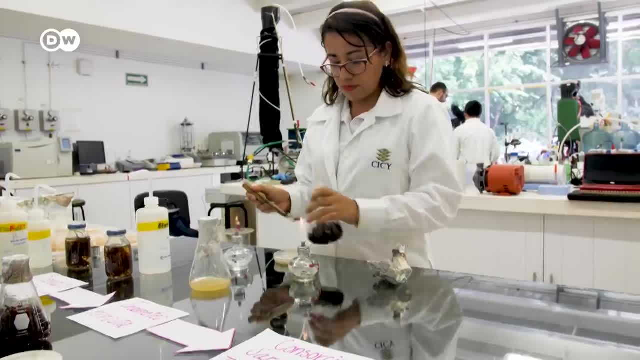 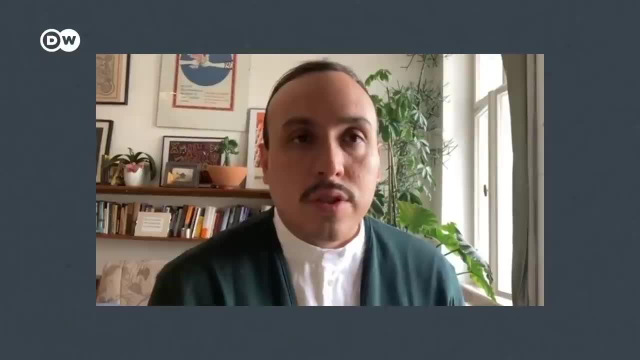 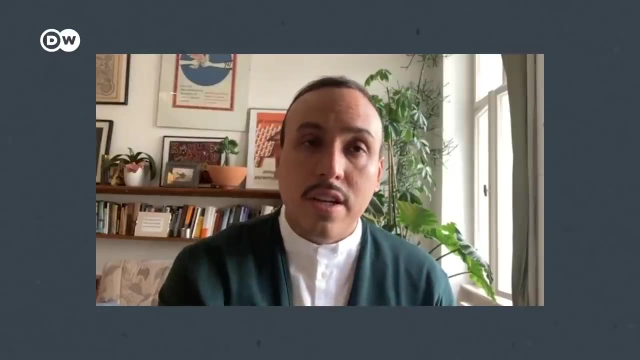 One promising use is fertilizer, something that dates back to the Roman Empire. Now it's being synthesized into extracts for large-scale use. We're able to turn it into different compounds that are applied Foliarly, so on the plant itself as a spray. 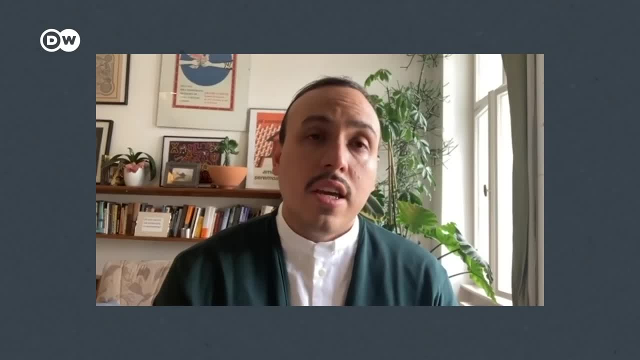 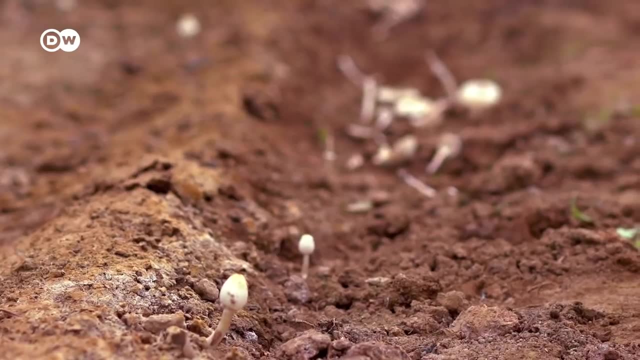 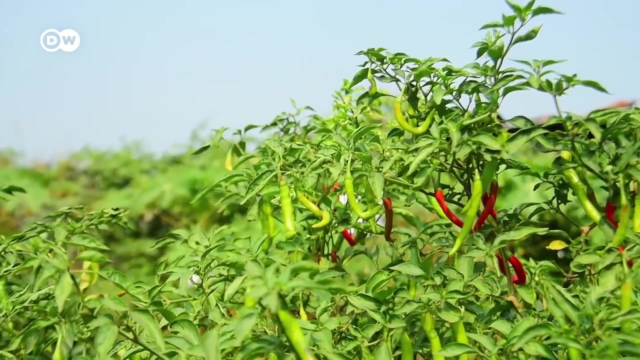 that can be applied directly into the land, either in liquid form or also in little granules. Nutrients in the fertilizer enrich the soil and induce processes in the plant that protect against pathogens. The result is more fruits and plants more resistant to stress and disease. 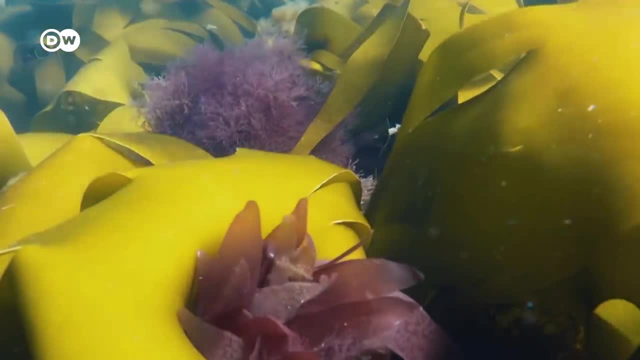 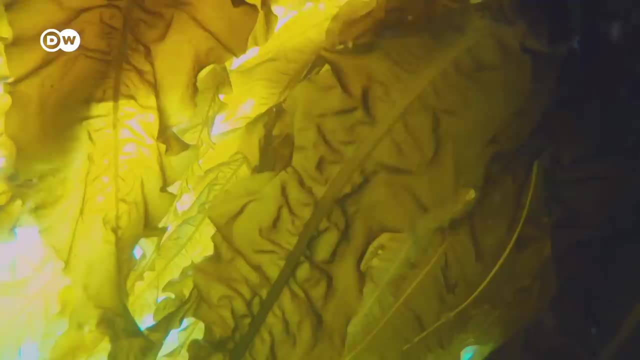 But the most direct way to use algae is also the simplest pure CO2 sequestration. Algae naturally falls to the ocean floor. when it dies. There it stores its captured CO2.. We can speed up this process If we want to enhance the amount of carbon. 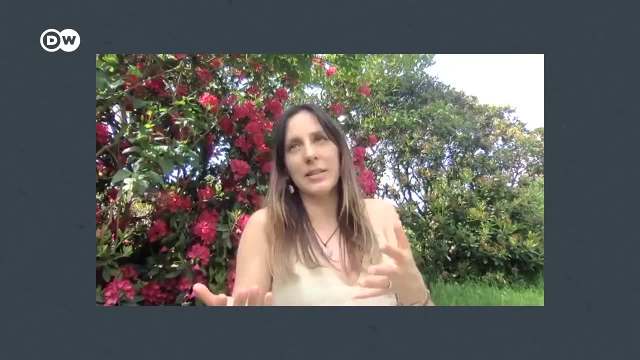 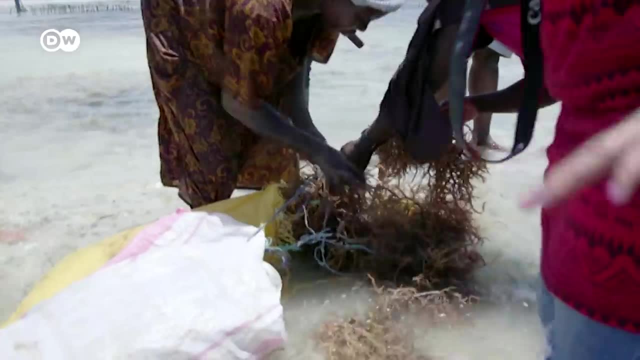 that is actually sequestered by this sargassum in this example, then we would actively need to, you know, bale it, compress it and actively sink it. This means adding weights or using a pump to send it to the bottom of the ocean. 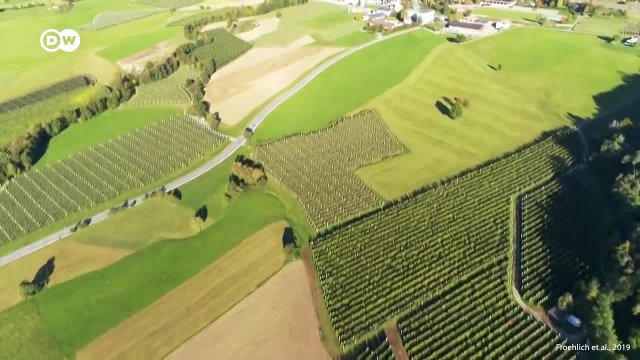 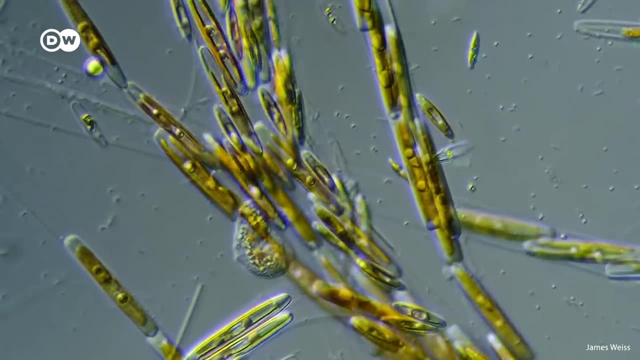 A recent study found that global agricultural emissions could be offset by using 2% of the ocean to farm and sink seaweed. So why haven't we been doing this already? The most widely farmed macroalgae kelp only grows attached to something. 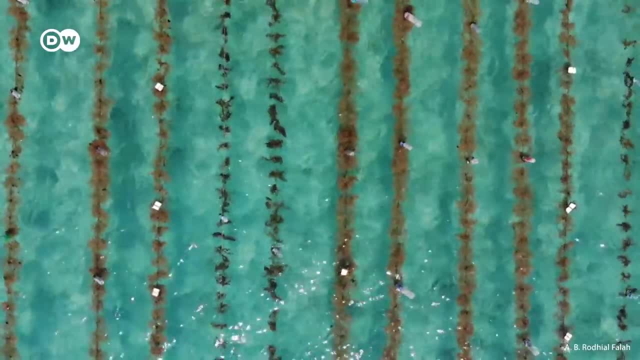 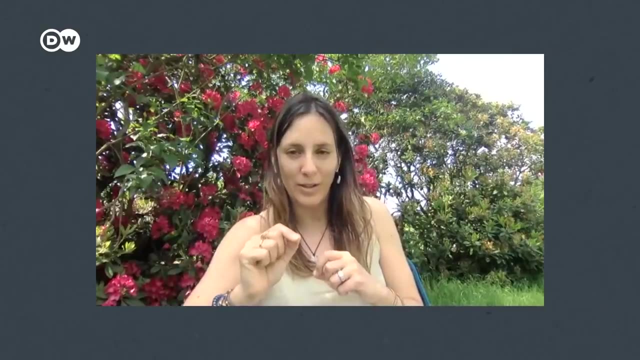 Some kelp farms are making headlines for sinking algae, but on a large scale it would require a lot of infrastructure. Here's where sargassum comes in. If you have a macroalgae that can grow everywhere floating in the ocean. 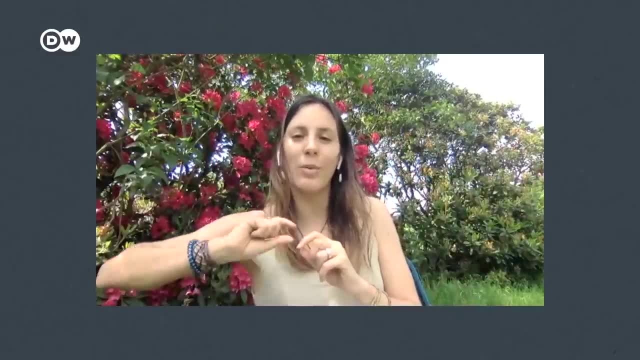 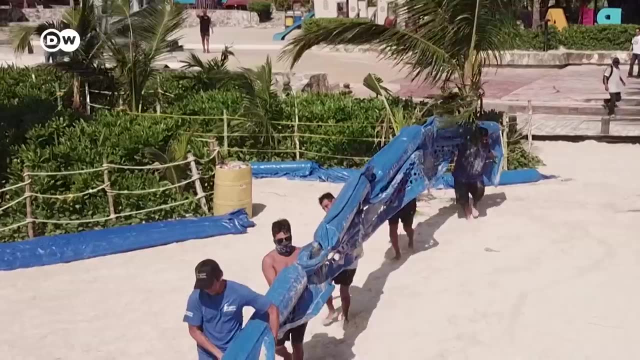 like phytoplankton does, but can sequester that carbon with a way higher efficiency than phytoplankton, then you have a winner, And that's sargassum. The technology to collect sargassum is already in use in affected areas. 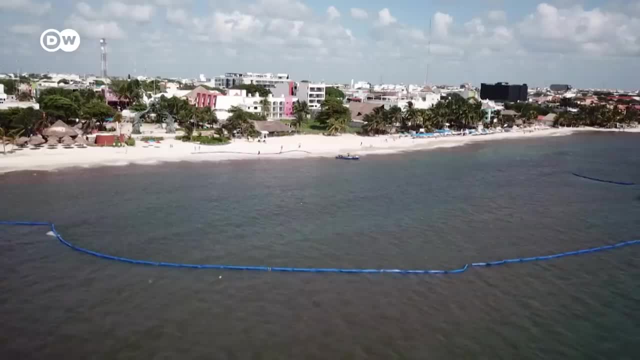 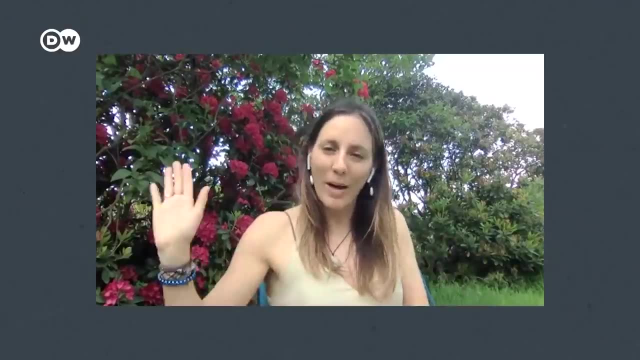 like Mexico, And people from a seaweed startup in the UK to the Mexican government are working on making it more efficient. This is not just something that people like me- you know biologists- should be looking at. This is something that the whole society should be looking at.